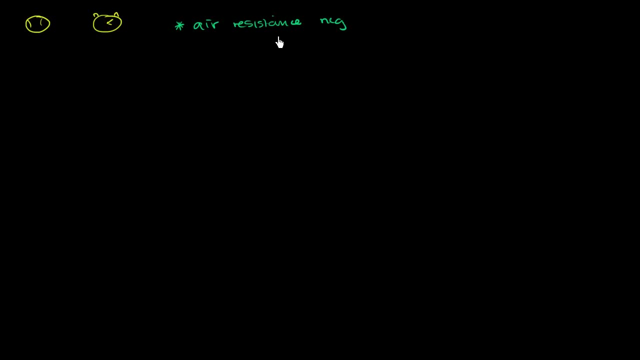 but we're going to assume for this projectile motion and really all of the future ones, or at least in the basic physics playlists- we're going to assume that air resistance is negligible And what that does for us is that we can assume that the time up. 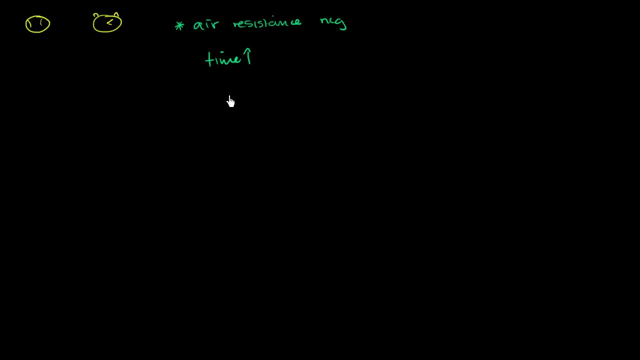 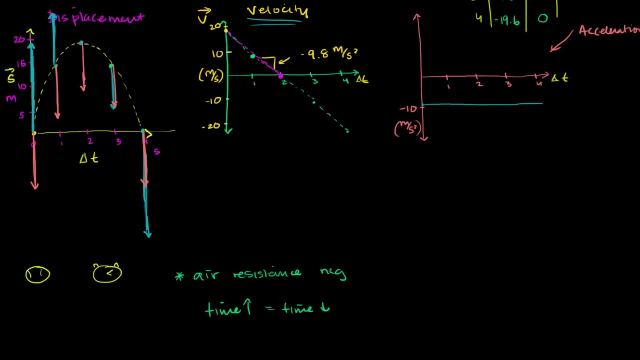 that the time for the ball to go up to its peak height is the same thing as the time that it takes to go down. If you look at this previous video where we plotted displacement versus time, you see after two seconds the ball went from being on the ground or, I guess, the thrower's hand. 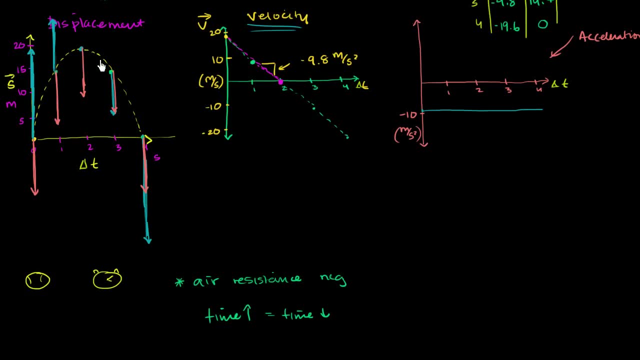 all the way to its peak. So that's the peak height and then the next two seconds. it took that same amount of time to go back down to the ground, which makes sense. Whatever the initial velocity is, it takes half the time to go to zero. 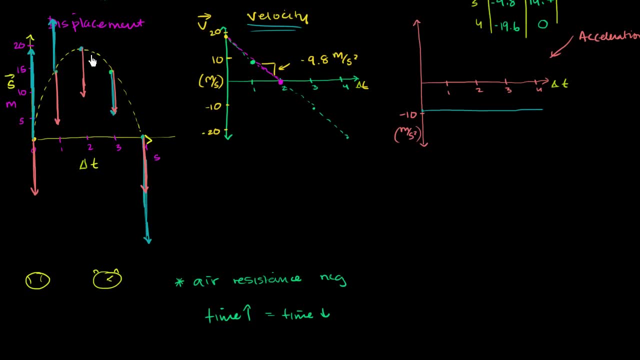 and then it takes that same amount of time to now be accelerated in the downward direction, back to that same magnitude of velocity, but now in the downward direction. So let's play around with some numbers here, just so we get a little bit more of a concrete sense. 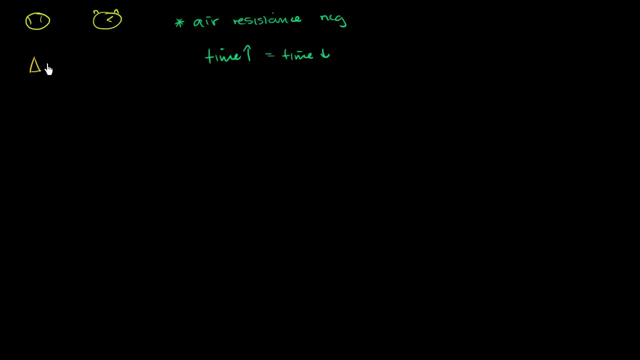 So let's say I throw a ball in the air and you measure using the stopwatch that the ball is in the air for five seconds. So how do we figure out how fast I threw the ball? Well, the first thing we can do is we can say: 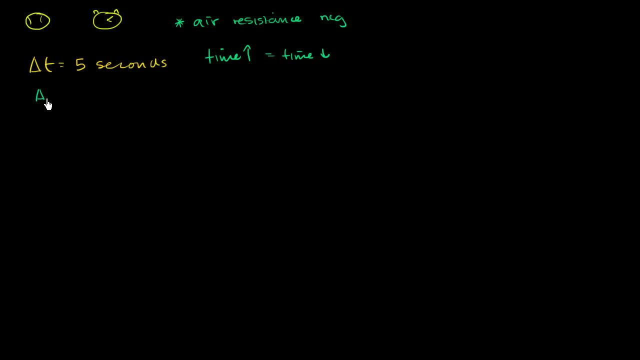 look, if the total time in the air was five seconds, that means that the time- let me write it well- that means that the change in time to go up during the first half of, I guess, the ball's time in the air. 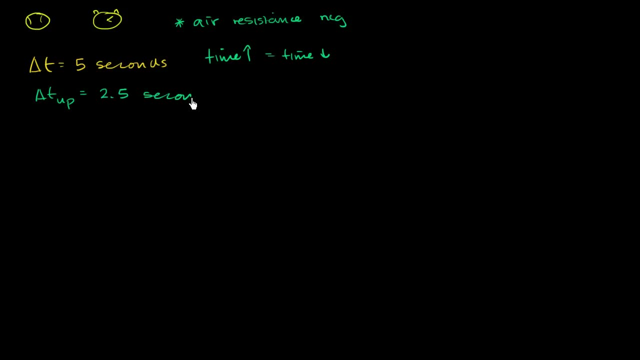 is going to be 2.5 seconds And which tells us that, over this 2.5 seconds, we went from from our initial velocity, whatever it was, we went from our initial velocity to our final velocity, which is a velocity of zero meters per second. 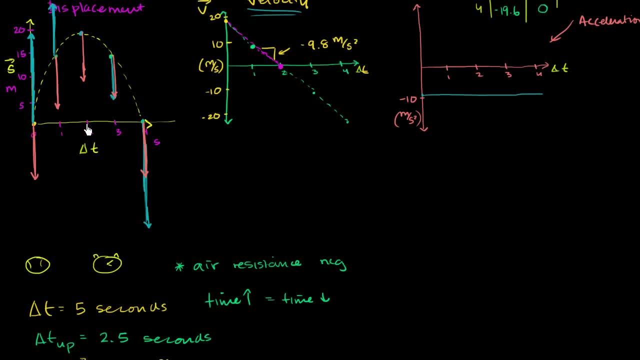 In the 2.5 seconds, and this isn't the graph for that example. this is the graph for the previous one. I the previous example where we knew the initial velocity, but in whatever that time is, you're going from your initial velocity to being stationary at the top. 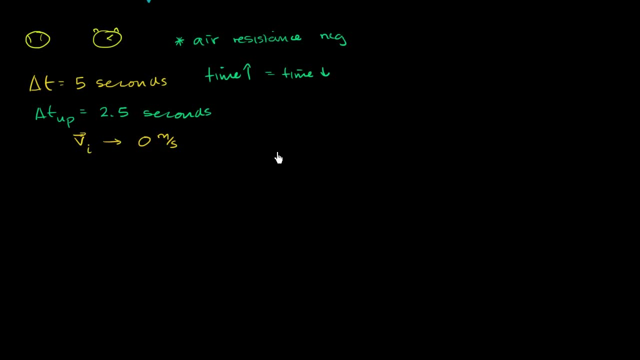 right when the ball is stationary and then starts getting increasing velocity in the downward, in the downward direction. So it takes 2.5 seconds to go from some initial velocity to zero seconds. So we do know what the acceleration of gravity is. We know that the acceleration 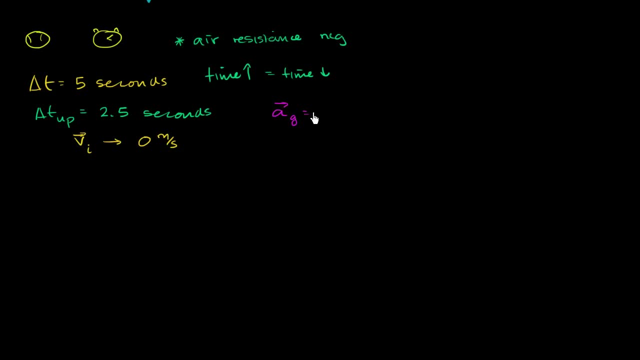 we know that the acceleration of gravity- here we're assuming it's constant, although it's slightly not constant, but we're going to assume it's constant if we're just dealing close to the surface of the earth- is negative 9.8 meters. 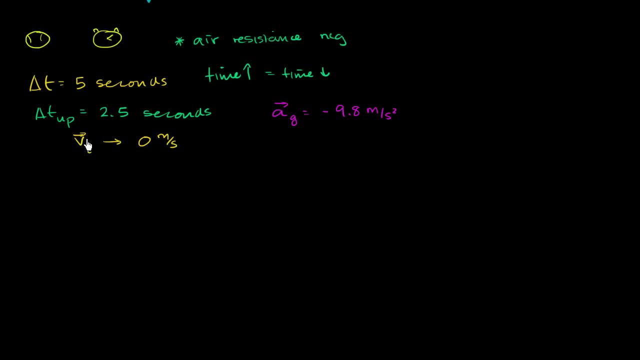 meters per second, squared. So let's think about it: This, our change in velocity, our change in velocity, our change in velocity is the final velocity minus the initial velocity, which, which is the same thing as 0 minus the initial velocity. 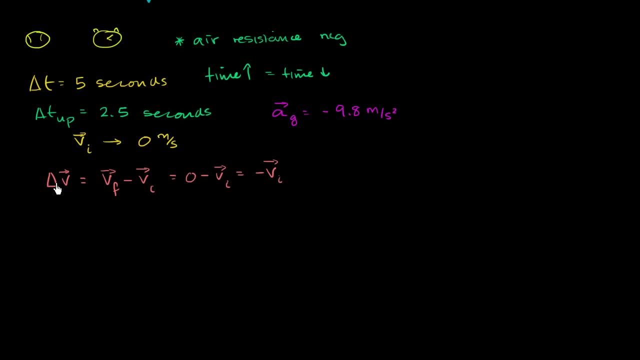 which is the negative of the initial velocity. And what's another way to think about change in velocity? Well, just from the definition of acceleration, change in velocity is equal to acceleration is equal to acceleration negative 9.8 meters per second squared times time. 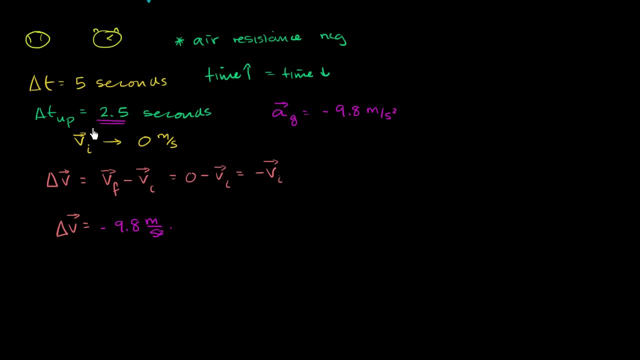 or times change in time, Our change in time. we're just talking about the first half of the ball's time in the air, So our change in time is 2.5 seconds times 2.5 seconds. So what is our change in velocity? 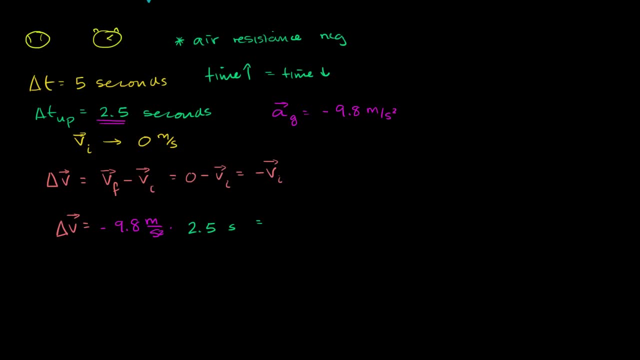 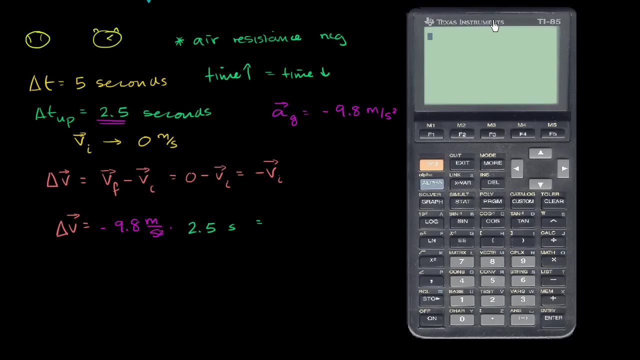 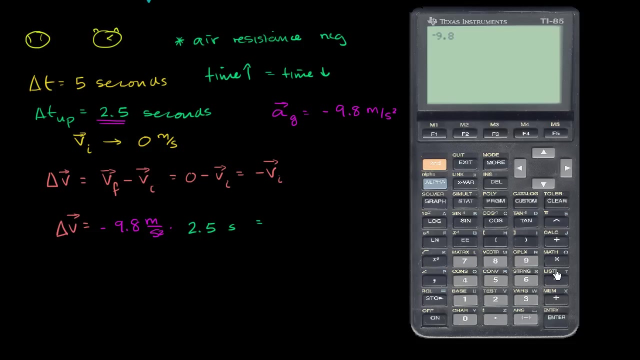 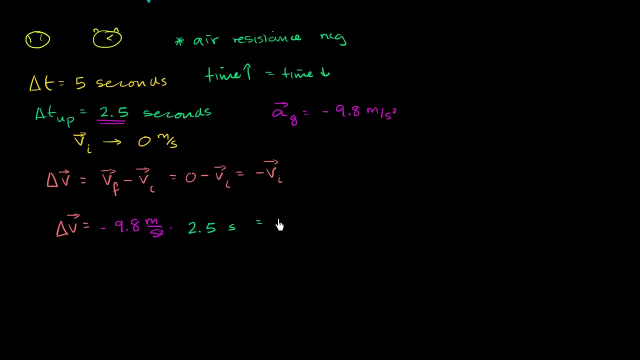 which is also the same thing as the negative of our initial velocity. Get the calculator out. Let me get my calculator. bring it onto the screen. So it is negative 9.8 meters per second. times 2.5 seconds, It gives us negative 24.5 meters per second. 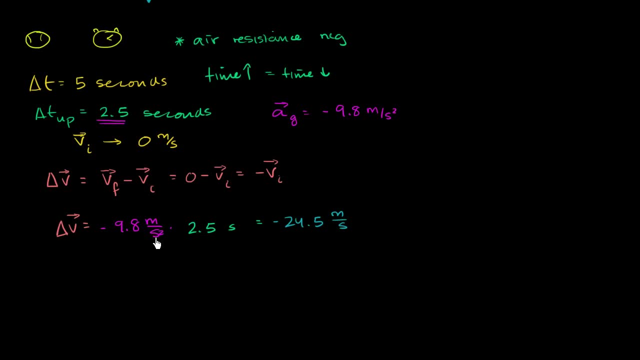 This second cancels out with one of the seconds in the denominator, so we only have one in the denominator now. so it's meters per second, And this is the same thing as the negative initial velocity. That's the same thing as our change in velocity. 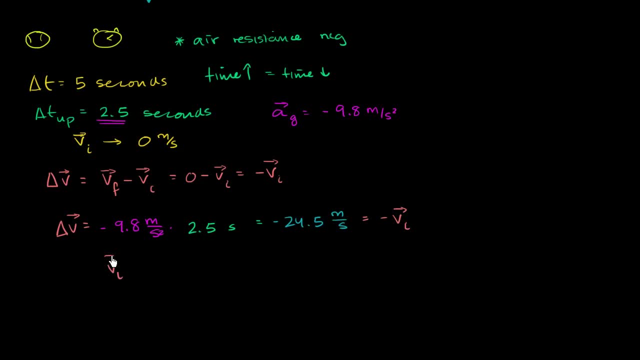 And so you multiply both sides by a negative. we get our initial velocity, So that, simply, we were able to figure out what our velocity was. So, literally, you take the total time in the air, divide it by 2, and then multiply that. 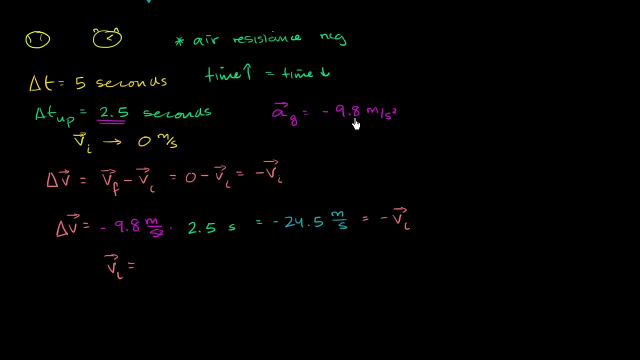 by the acceleration of gravity, And I guess you could take the absolute value of that, or you take the positive version of that, And then that gives you your initial velocity. So your initial velocity here is literally 24.5 meters per second. 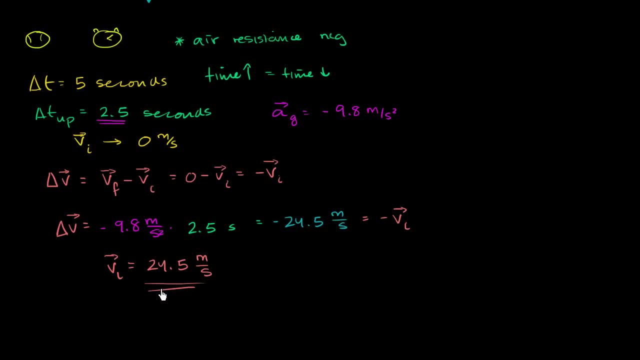 And since it's a positive quantity, it is upwards in this example. So that's my initial velocity. So we already figured out part of this game, the initial velocity that I threw it upwards And that's also going to be we're. going to have the same magnitude of velocity when the ball is up. So we're going to have the same magnitude of velocity when the ball is up, So we're going to have the same magnitude of velocity when the ball is about to hit the ground. 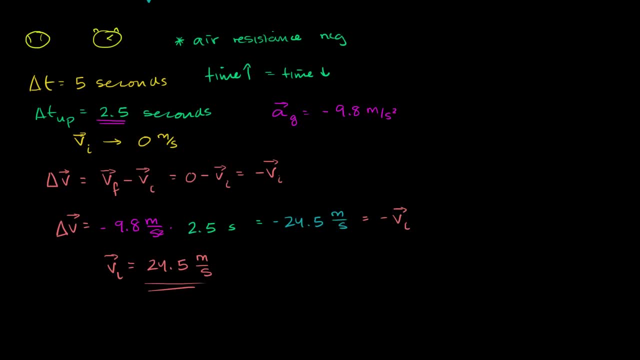 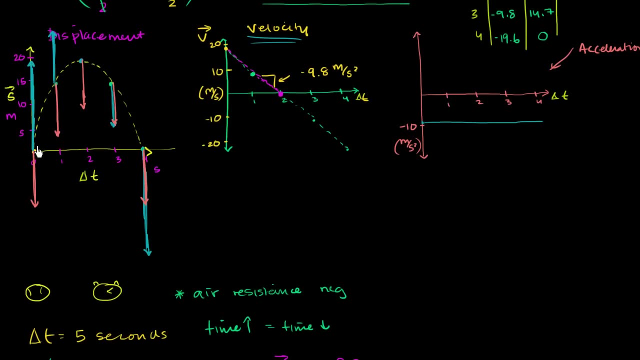 although it's going to be in the other direction. So what is the distance? or, let me make it clear, what is the displacement of the ball from its lowest point right when it leaves your hand all the way to the peak? Well, we just have to remember. 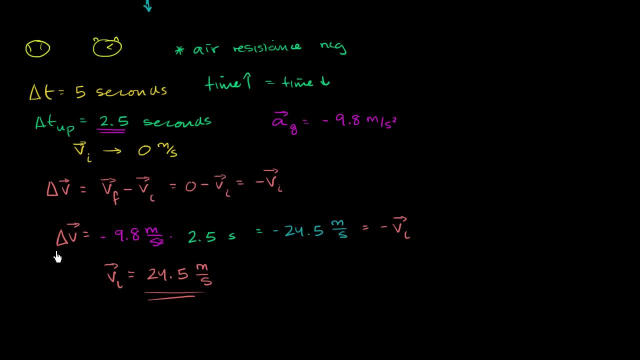 And once again, all this comes from very straightforward ideas: Change in velocity is equal to acceleration times. change in time. And then the other simple idea is that displacement is equal to acceleration times. change in time. And then the other simple idea is that displacement is equal to acceleration times. change in time. 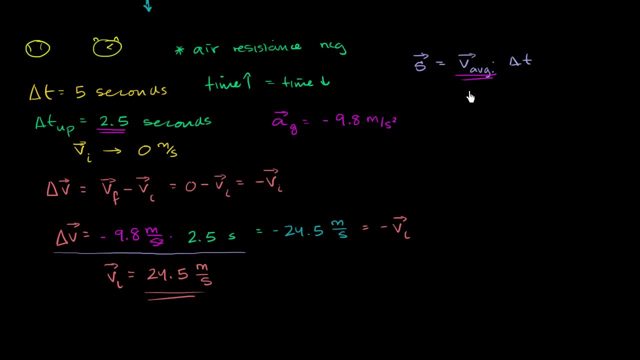 Now what is our average velocity? Our average velocity is your initial velocity plus your final velocity divided by 2, if we assume acceleration is constant. So it's literally just the arithmetic mean of your initial and final velocities. So what is that? 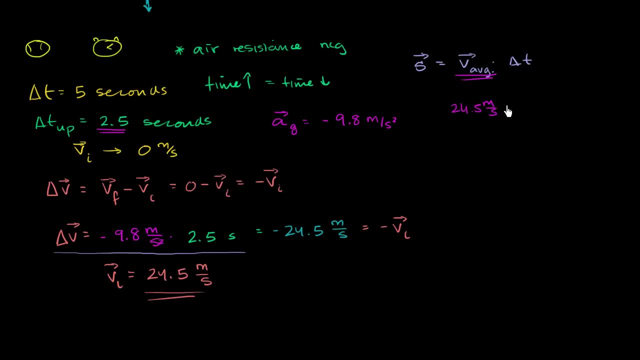 That's going to be 24.5 meters per second Plus. what's our final velocity In this situation? remember, we're just going over the first 2.5 seconds, So our final velocity is, once again, 0 meters per second. 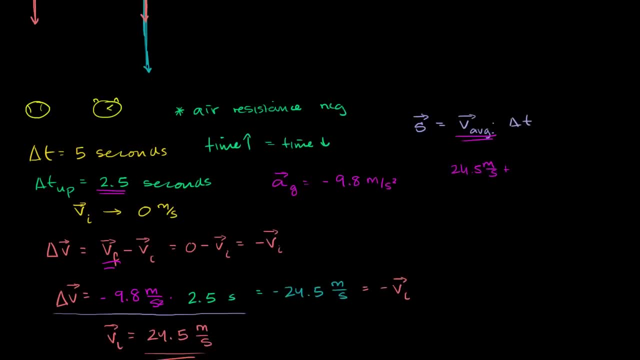 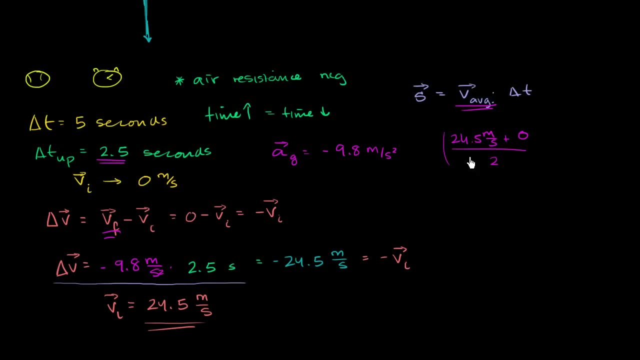 We're just talking about when we get to this point right over here. So our final velocity is just 0 meters per second, And we're just going to divide that by 2. This will give us the average velocity, And then we want to multiply that times 2.5 seconds. 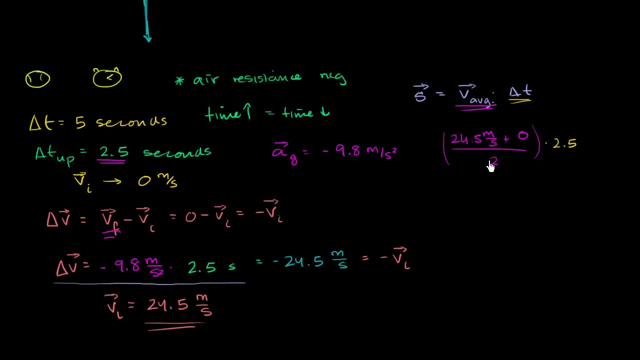 So we get this part right over here: 24.5.. 24.5 divided by 2.. We can ignore the 0. That still is 24.5.. That gives us 12.25 times 2.5.. 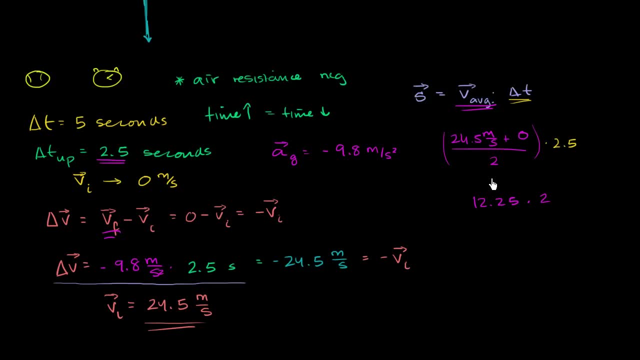 And remember this right over here is in seconds. Let me write the units down. So this is 12.25 meters per second times 2.5 seconds. And just to remind ourselves, we're calculating the displacement over the first 2 and 1.